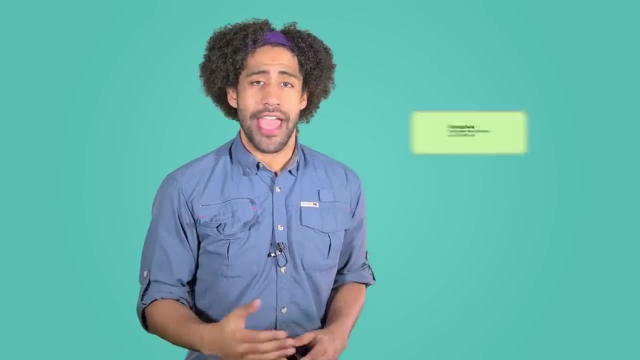 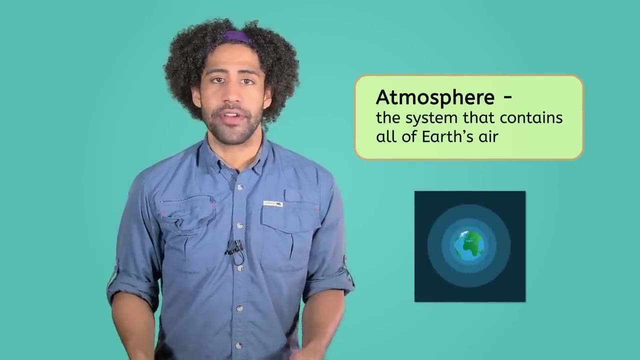 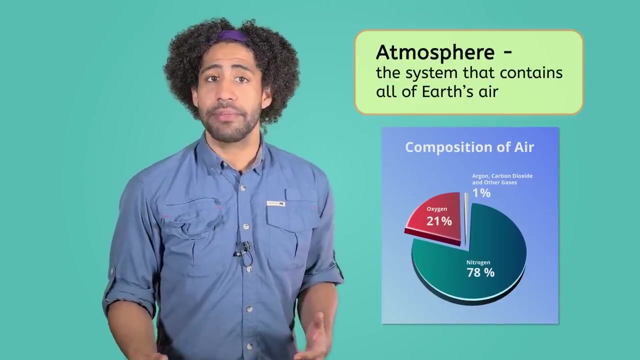 In our lesson on Earth's spheres, we learned that the atmosphere is a system that contains all of Earth's air or the gases that surround our planet. Our atmosphere is made up of a combination of gases including 78% nitrogen, 21% oxygen and trace amounts of others, such as carbon dioxide. 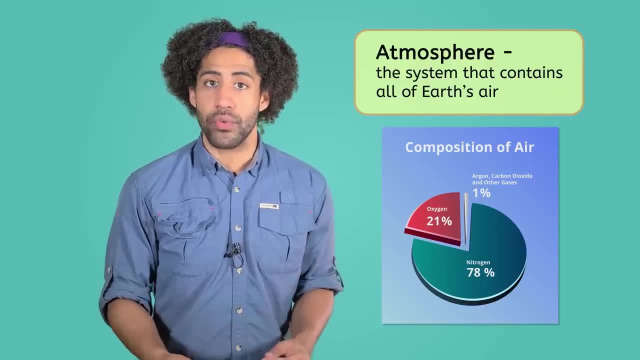 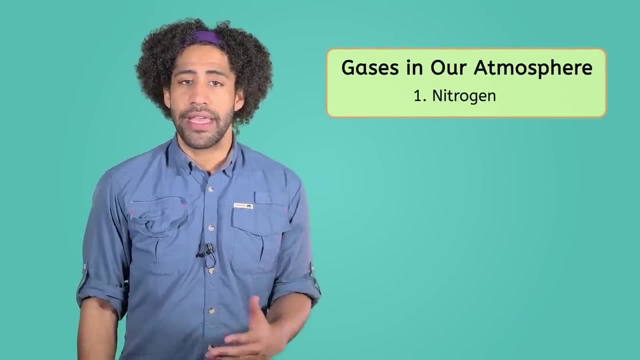 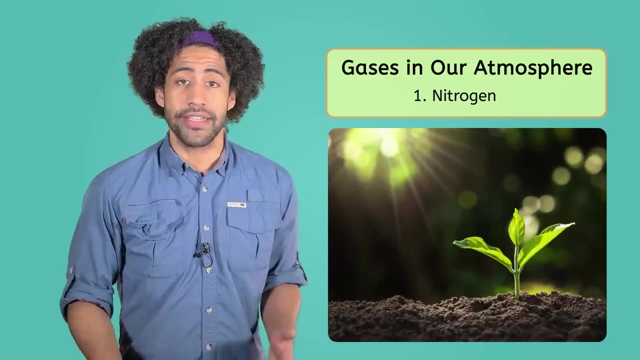 and water vapor. These gases play an important role in supporting life on our planet. Most of the gas in our atmosphere is nitrogen. It's essential for the nitrogen cycle, which transforms the gas into a more usable form that nearly all plants need to grow properly. 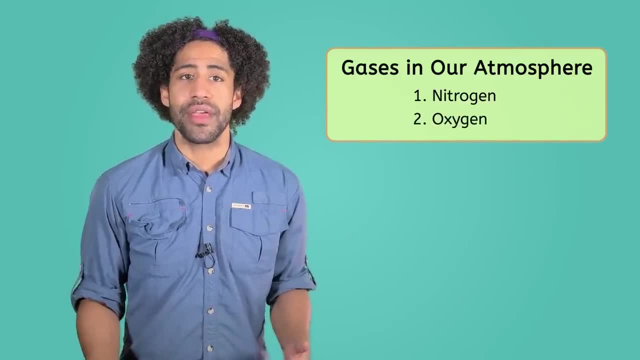 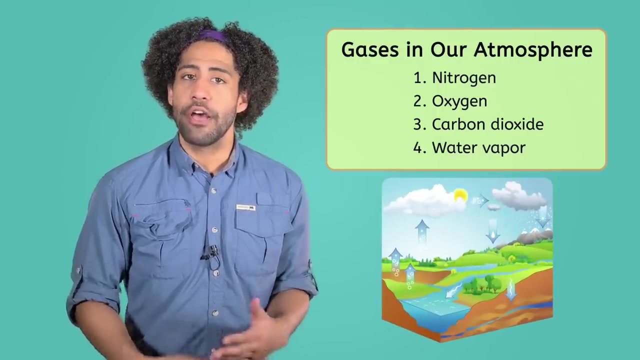 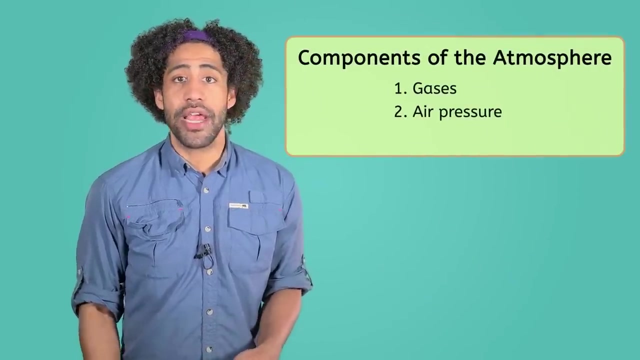 Oxygen is necessary for all living things to breathe and survive. Carbon dioxide helps regulate the Earth's temperature and is necessary for photosynthesis. Water vapor is a key part of the water cycle and helps regulate global temperatures, weather and climate. Along with gases, air pressure and temperature are also important components of the atmosphere. 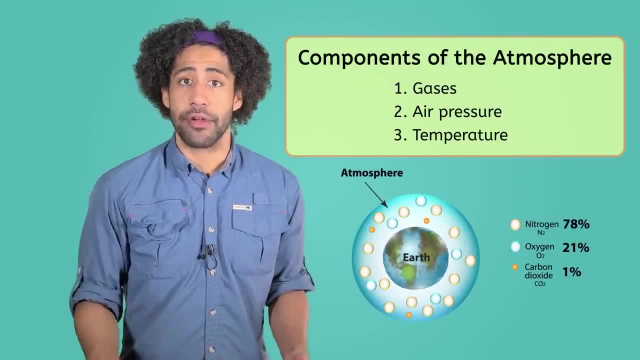 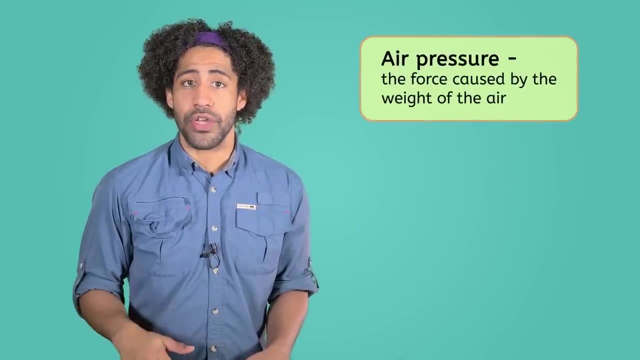 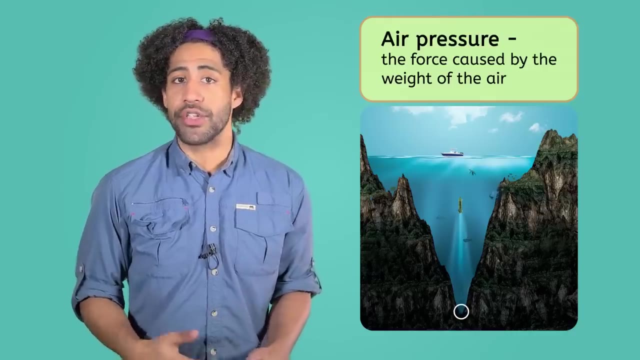 We see this same blend of gases throughout the atmosphere, but air pressure and temperature change as we go higher up. Air pressure is the force caused by the weight of the air. In our lesson on Earth's oceans, we learned that the weight of the water adds to the pressure. 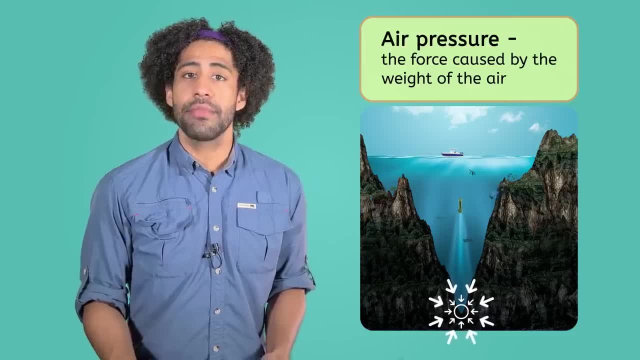 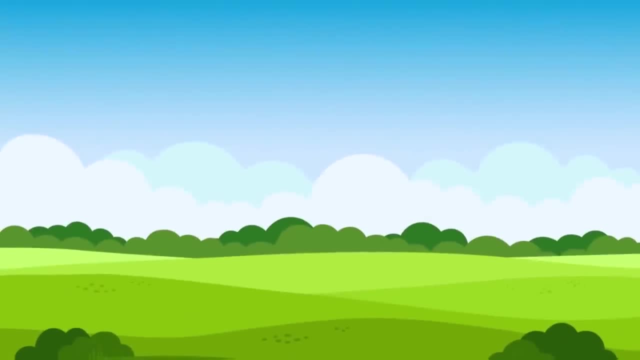 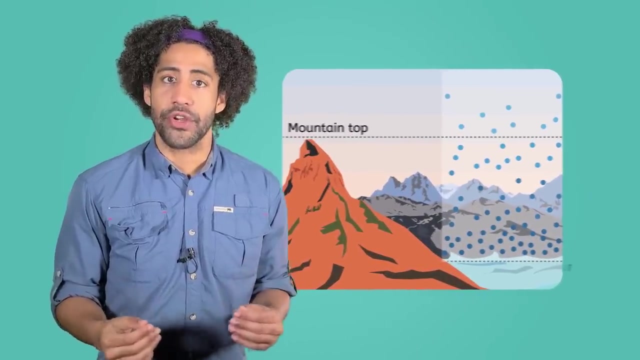 the deeper we travel towards the ocean floor. Similar to the ocean floor, the Earth's surface is where the air pressure is the greatest. The gravitational pull of the Earth attracts the molecules of air downward toward the surface, keeping our atmosphere in place. This pull results in more of these fast-moving atoms bumping into each other closer to the Earth's surface. Air pressure decreases as you travel higher up because there are fewer gas molecules bumping into each other. Temperature varies or changes in different layers of the atmosphere. The atmosphere is made up of five main layers. Remember the zones of the ocean. 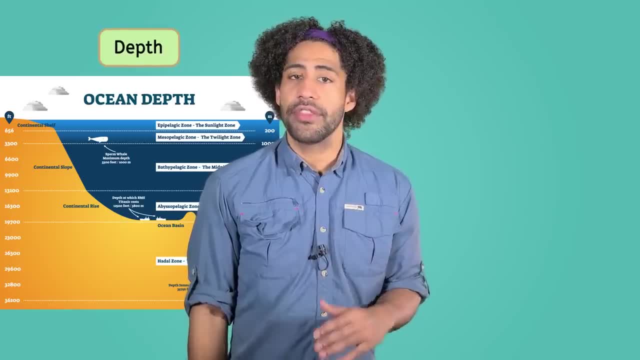 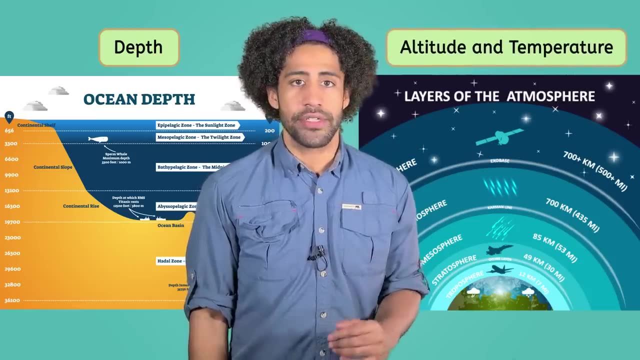 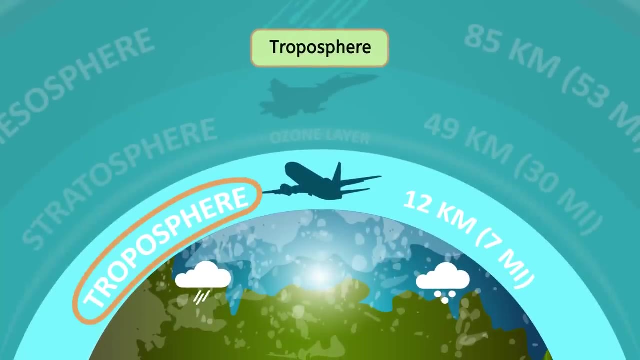 They changed based on the depth below the ocean's surface, The layers of the atmosphere, however, based on two things: altitude, or the height above the ground, and temperature. The first layer is the troposphere, which is closest to the Earth's surface. 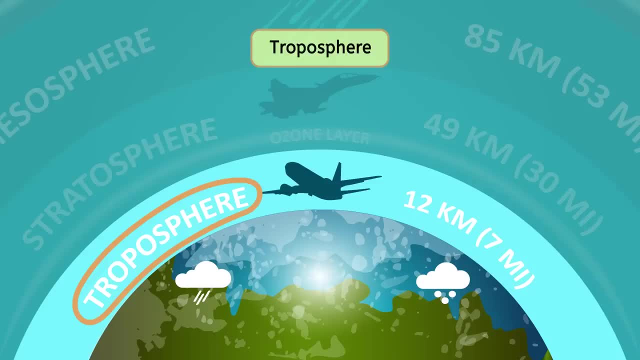 This is where we live, and it extends from the ground to about 12 kilometers high, that's a few kilometers above the tallest mountain in the world, Mount Everest. This layer contains all the air that living things need to survive, and it's where most 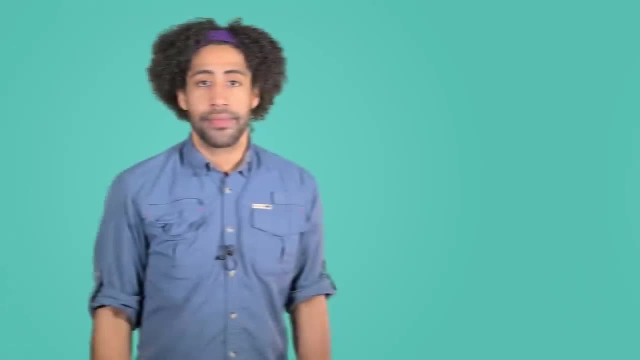 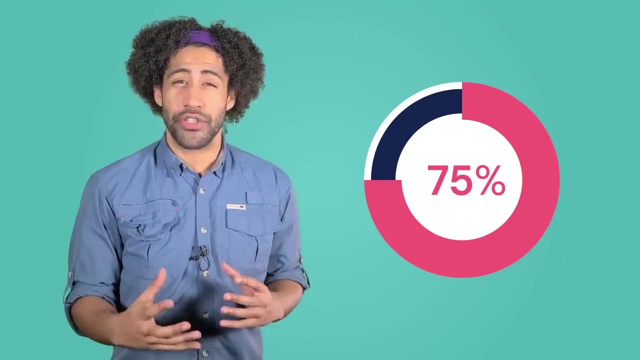 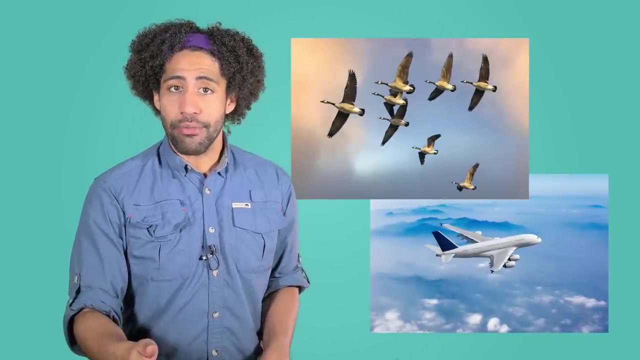 of our clouds and weather are formed. The troposphere contains most of the gas in our atmosphere, about 75%. That dense concentration of gases creates a stable layer that supports the flight of birds and planes. Air pressure is at its highest at the ground and decreases as we travel away from the surface. 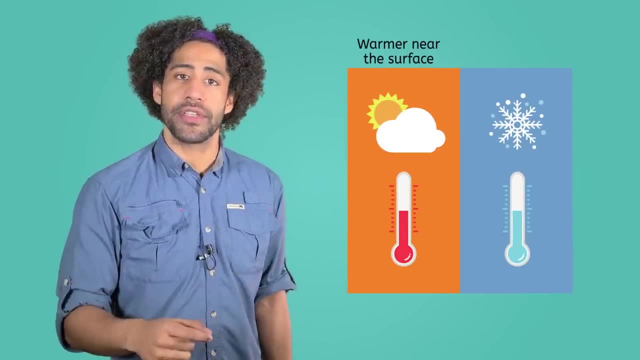 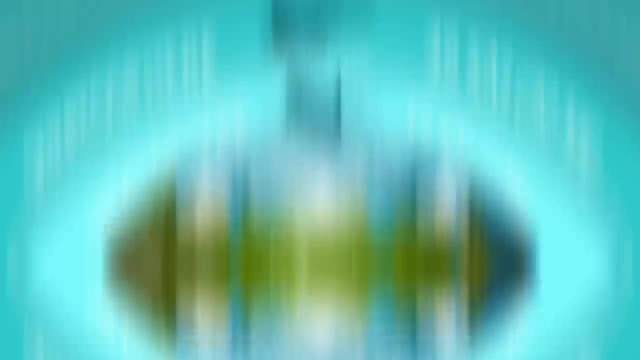 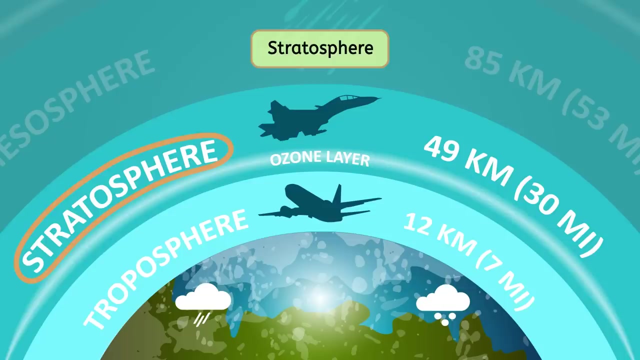 The temperature in this layer is warmer near the surface and colder as we climb. However, this isn't the case for every layer. It's the atmosphere. The next layer is the stratosphere. It starts from the top of the troposphere and goes 50 kilometers high. 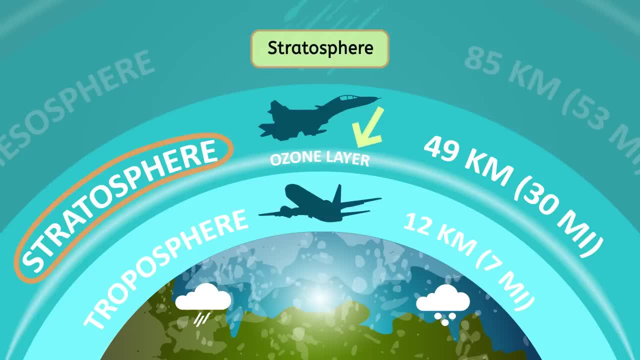 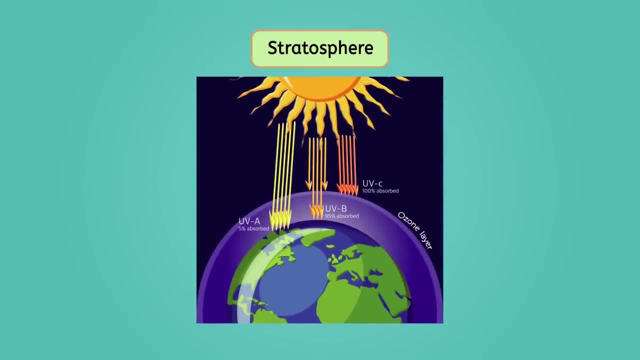 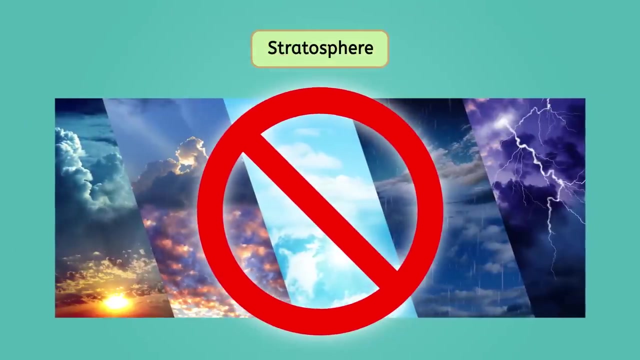 The stratosphere is home to the ozone layer. This layer is characterized by a high concentration of molecules that absorb the most harmful ultraviolet radiation from the sun. That energy is then turned into heat, Because heat rises and there is no weather or wind to circulate the molecules, like in 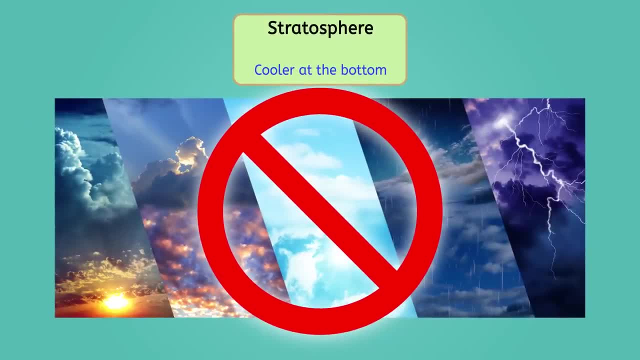 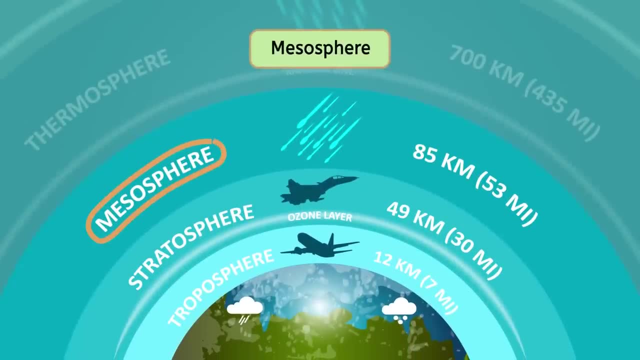 the troposphere. We find the cooler temperatures at the bottom of the stratosphere and warmer temperatures near the top. The mesosphere is above the stratosphere between 50 and 80 kilometers high. It's very cold and the air is thin. 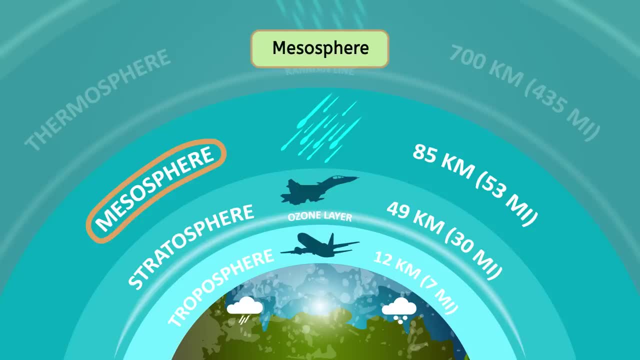 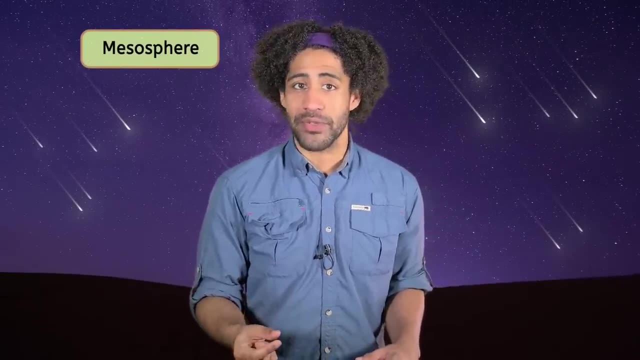 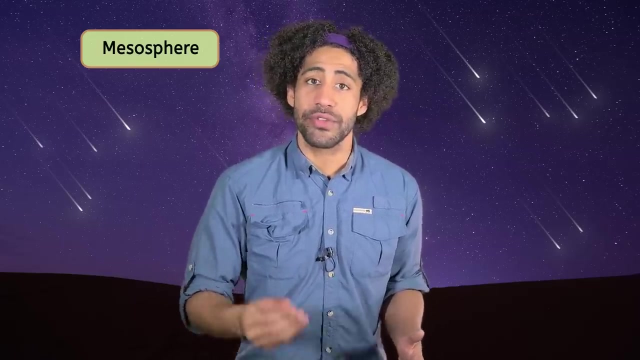 But there are enough gases in this layer to cause something pretty special: Meteor showers, sometimes referred to as shooting stars. They happen when small space rocks enter Earth's atmosphere. Once they reach the mesosphere, they burn and glow across the sky due to the friction. 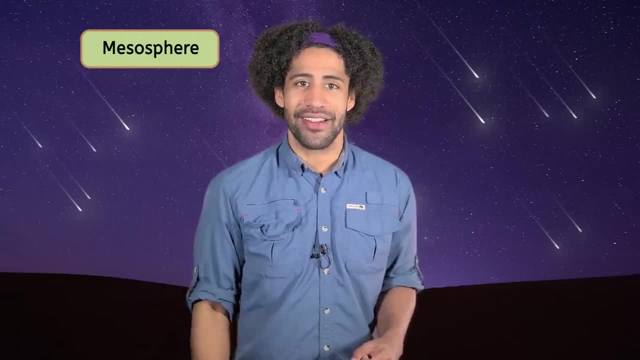 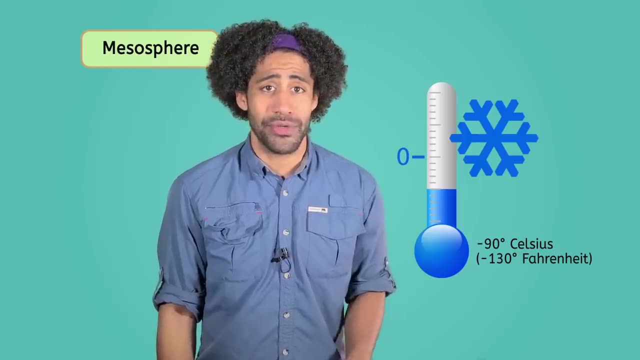 and heat generated as they hit the gases in this layer. The mesosphere contains some of the coldest temperatures in our atmosphere, with an average temperature well below zero. We'll also find a bit of water vapor here, which forms noctilucent clouds. 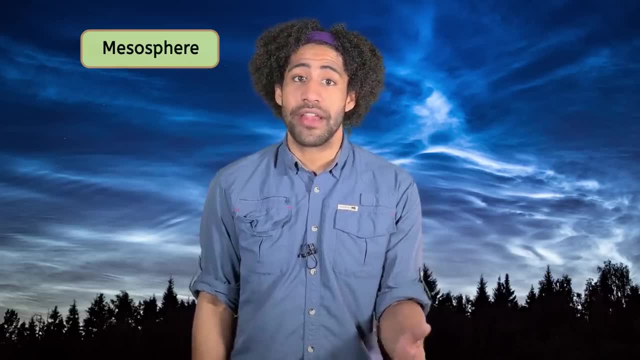 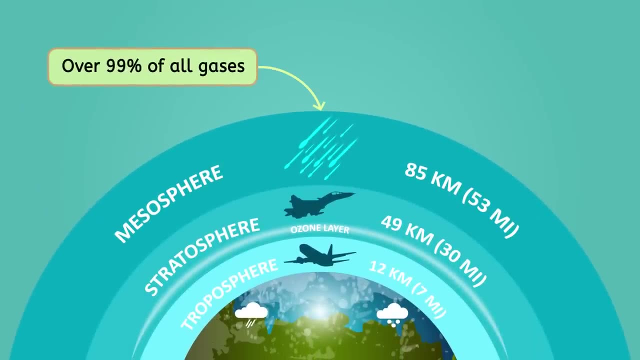 These are the highest clouds in the atmosphere and can be seen without a telescope under certain conditions. It's important to note that the atmosphere in the stratosphere is very cold. It's important to note that over 99% of all the gases in our atmosphere are found in. 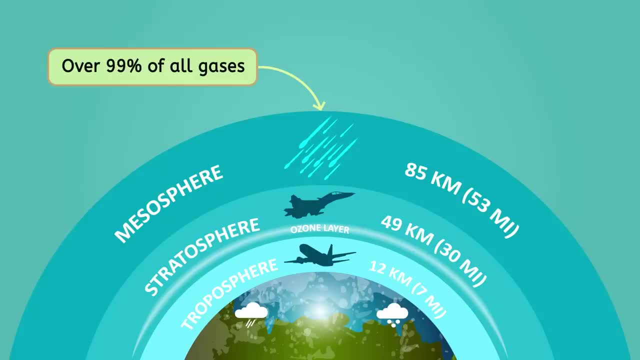 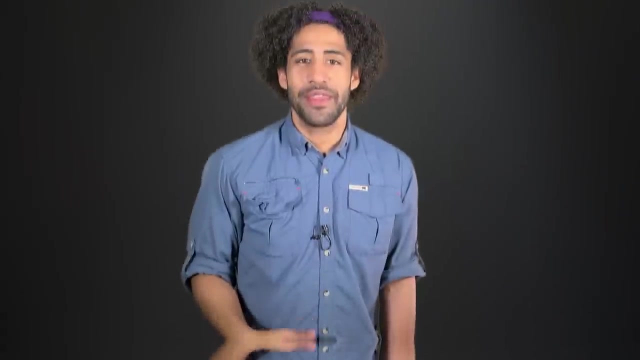 these first three layers closest to the Earth? What does that tell you about the distance between gas molecules and the two outer layers? Pause the video here and record your answer in your guided notes. The outer layers of the atmosphere are huge, but they're mostly empty space. 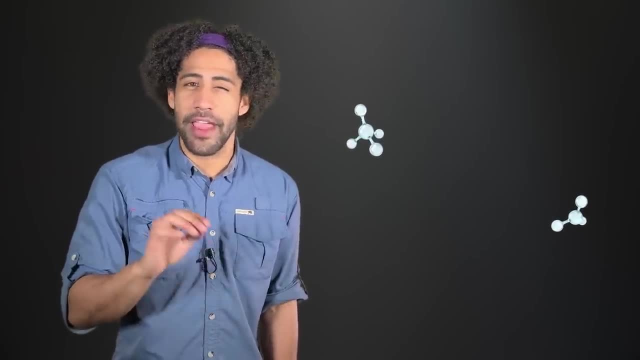 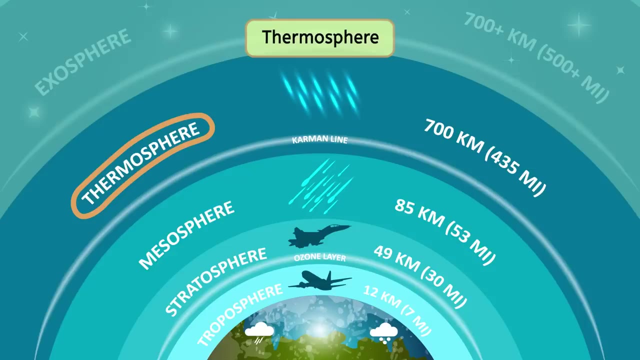 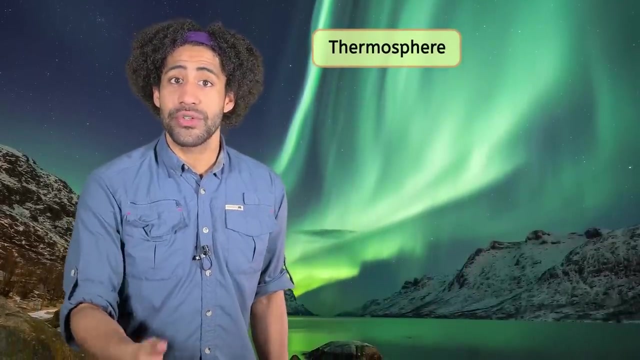 There are still some molecules in these layers, they're just very far apart. The thermosphere is above the mesosphere from 80 to 700 kilometers high. This is where the northern and southern lights, or the auroras, happen. They occur due to solar particles interacting with the gases in this layer. This layer is also where we'll find the International Space Station orbiting the Earth. The temperature patterns in the thermosphere are similar to the temperature patterns in the atmosphere. The thermosphere is above the mesosphere from 80 to 700 kilometers high. The stratosphere is above the mesosphere, getting warmer as you go higher. There are very few molecules here, but they can get extremely hot, up to 4500 degrees Fahrenheit. They're very far apart and rarely bump into each other, so it would still feel very cold. in this part of the atmosphere. Finally, the exosphere is the outermost layer, from 700 to 10,000 kilometers high. This is where we'll find most of the satellites orbiting Earth. The gases in this layer are mostly hydrogen and helium, and they're very far apart from. each other, Particles from this layer often escape into space. So, with all these layers, where exactly is the edge of outer space? 10,000 kilometers sounds really far. Do we really need to go that far to reach space if the Earth's atmosphere is already? 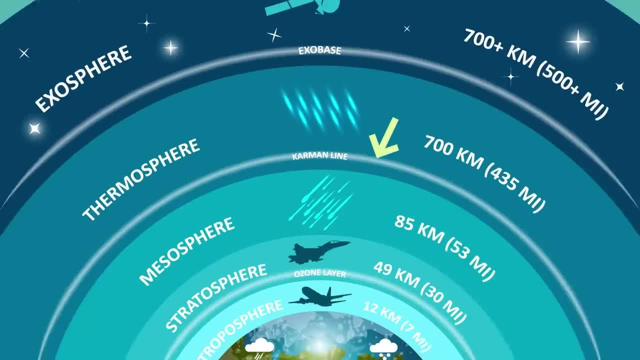 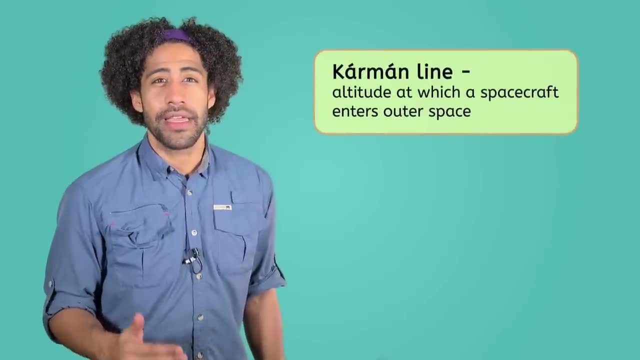 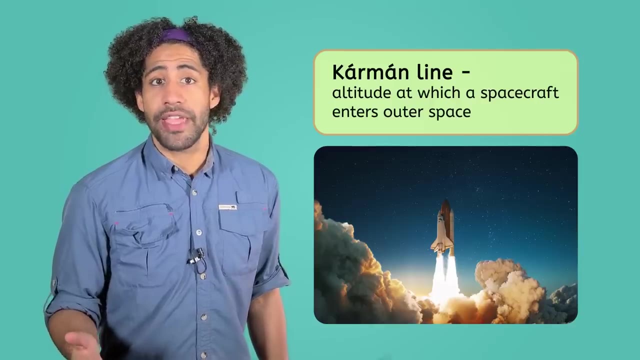 so thin by that point. Scientists use 100 kilometers above the Earth's surface as a reference point that they call the Karman line. The Karman line is the altitude at which a spacecraft enters outer space. Why 100 kilometers? Most of the gases in the atmosphere are found within 100 kilometers of the Earth's surface. 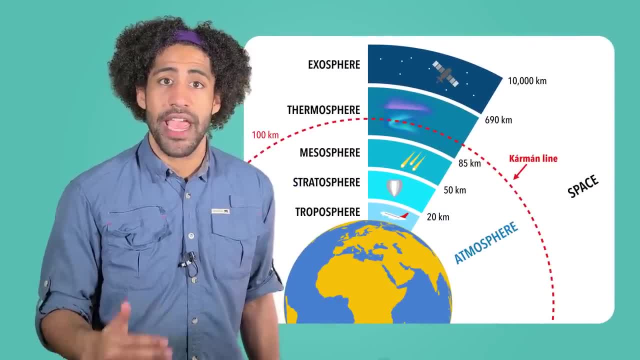 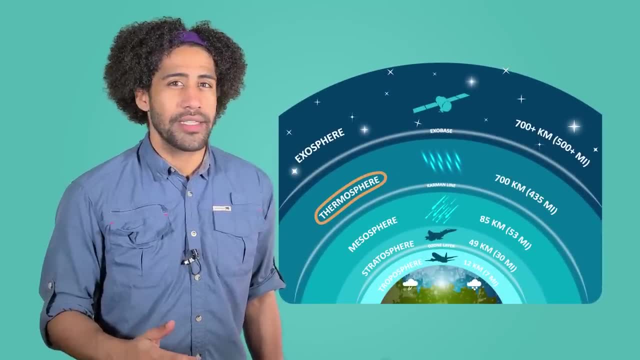 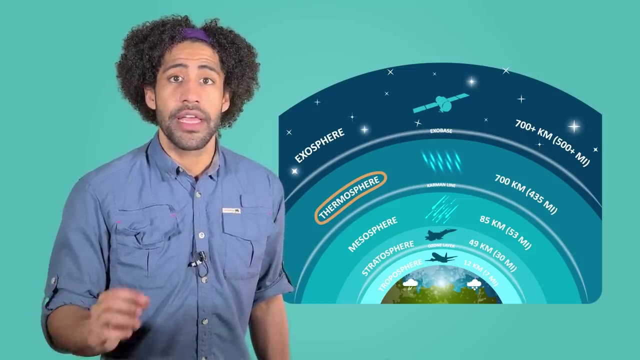 so this is considered the boundary between Earth's atmosphere and space. That means space technically begins in the thermosphere. That's right. So why is the exosphere considered part of Earth's atmosphere? Even though the exosphere contains very few molecules, there are still more than there. 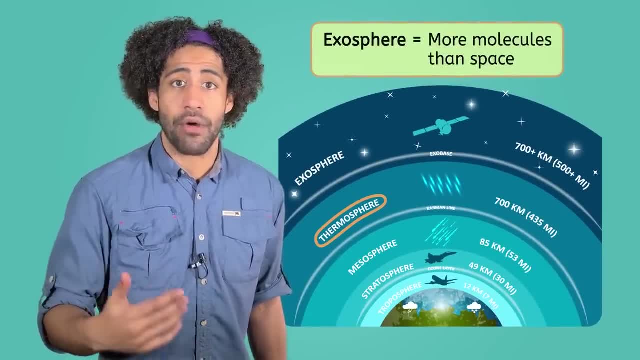 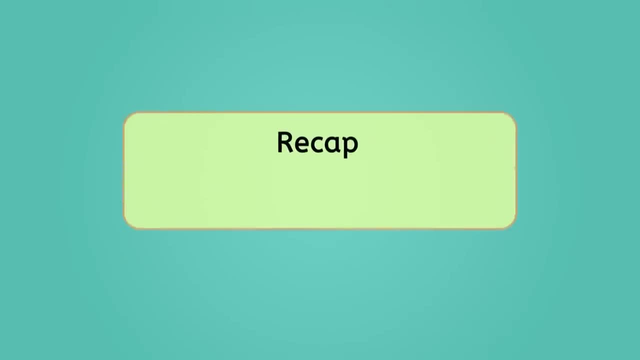 are in space. Therefore it's part of our atmosphere and a transition zone between the upper atmosphere and space. So let's go over what we learned today. We now know that gases, air pressure and temperature are all important components of Earth's atmosphere. 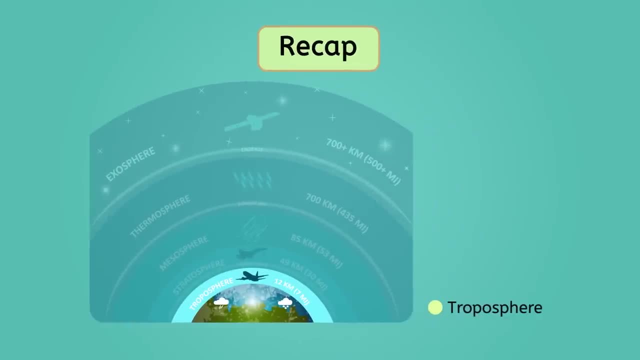 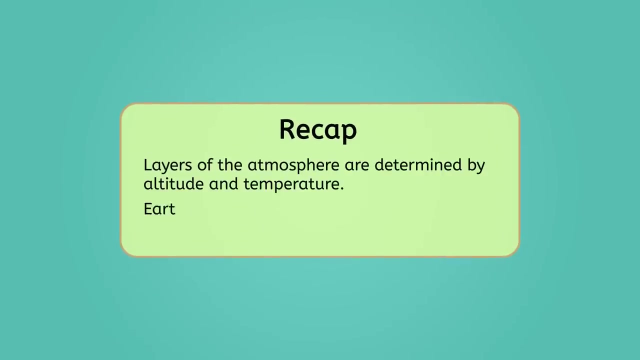 The five layers of the atmosphere are the troposphere, stratosphere, mesosphere, thermosphere and exosphere. The layers of the atmosphere are determined by altitude and temperature. Lastly, Earth's atmosphere is essential for supporting life on our planet.